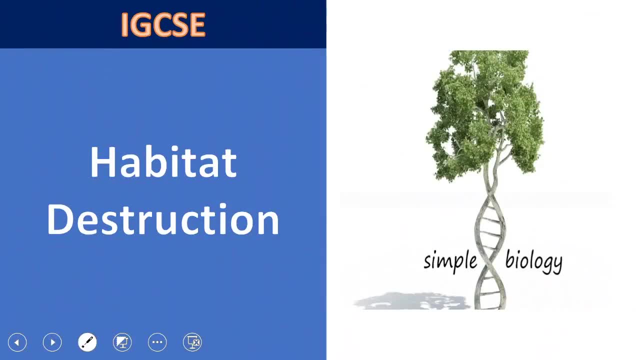 This is Symbol Biology and Habitat Destruction. Many habitats are destroyed by humans to make space for other economic activities or by pollution from these activities. Consequently, the biodiversity of many places is decreasing. This interrupts food chains and food webs and means that more species may die because their prey is just gone. So what are the causes of? 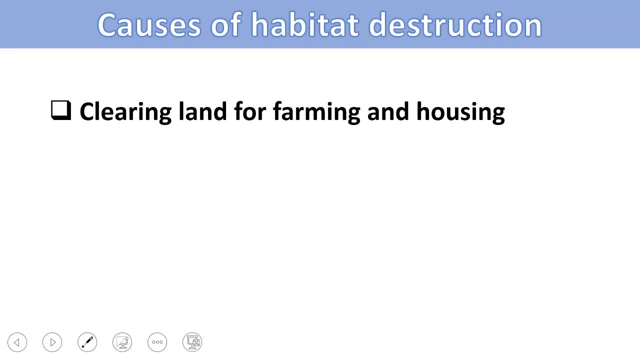 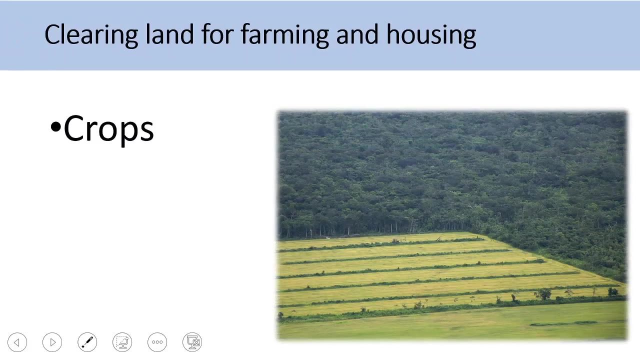 habitat destruction- The first on the list. clearing land for farming and housing, natural resource extraction and marine pollution. So let's start with clearing land. Clearing land for growing crops: We need to grow crops for our food and this needs to. 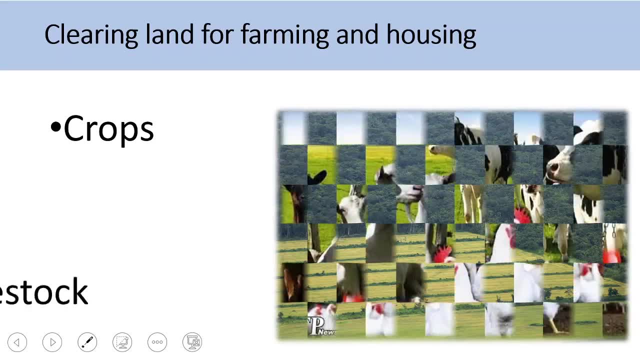 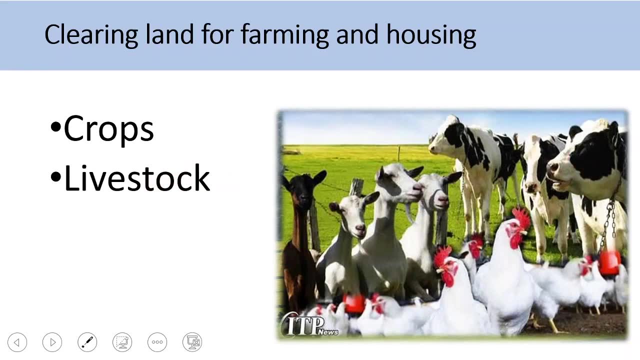 have more space for these crops. Also, the crops are grown for as a food for our livestock. We need to grow crops for our livestock. We need to grow crops for our livestock. We like to have meat and having meat. this means you have to raise animals that produce meat. 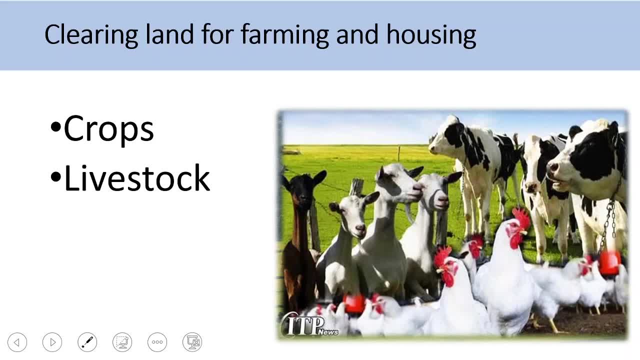 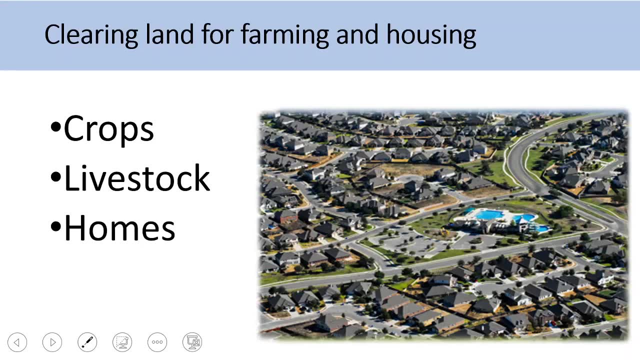 and these animals need food, and producing food for them requires land. The great demand for housing is another reason for clearing land. The human population is increasing, so we have to meet this demand by making more homes for our animals. So we need to have more land for our animals. So we need to have more land for our animals. So 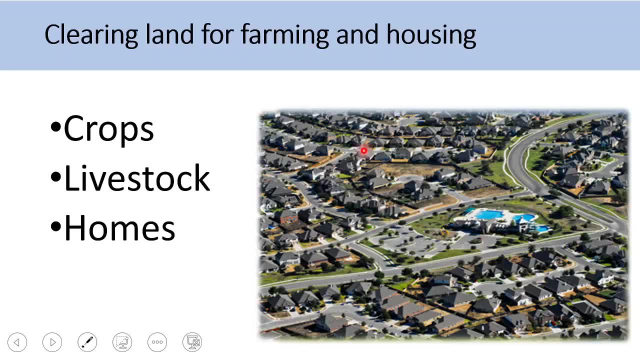 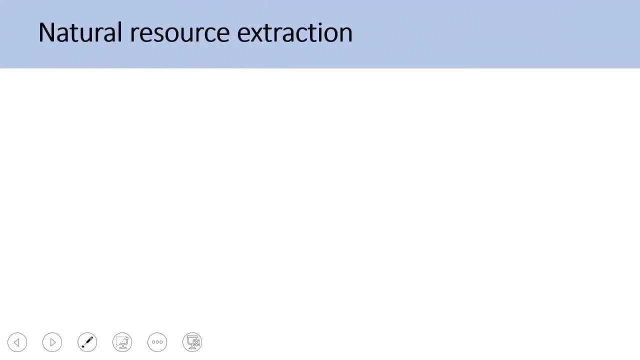 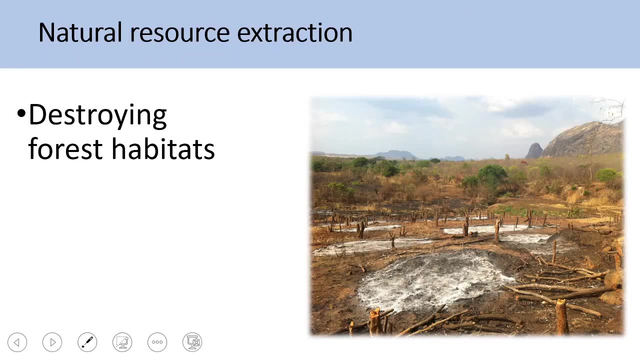 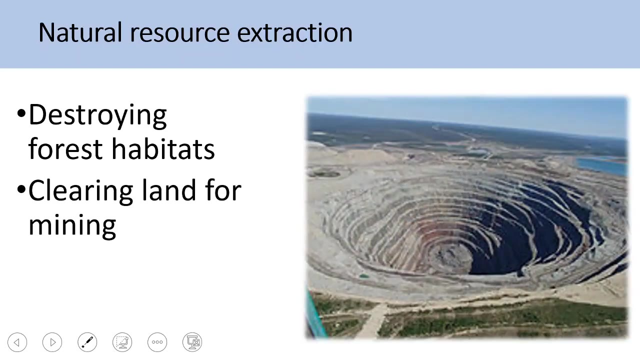 we need to have more land for our animals, So clearing land for mining. It's true that the minerals are deep in the underground, so it's good for us to Sleeping. horrible conditions, So stupid Sauce load. we need to clean land and maintain it, But when we're in außer Teil, we need more. So the decision is to isolated land and play the same. So the decision is to isolated land and play the same. 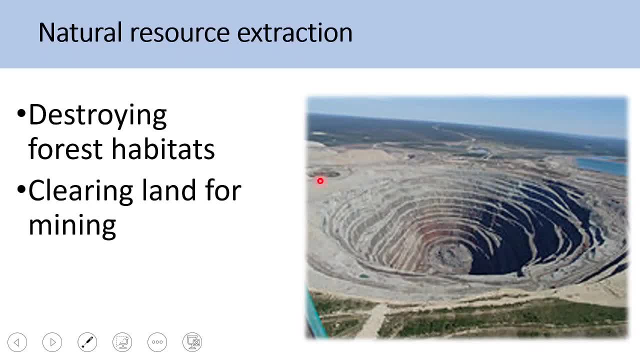 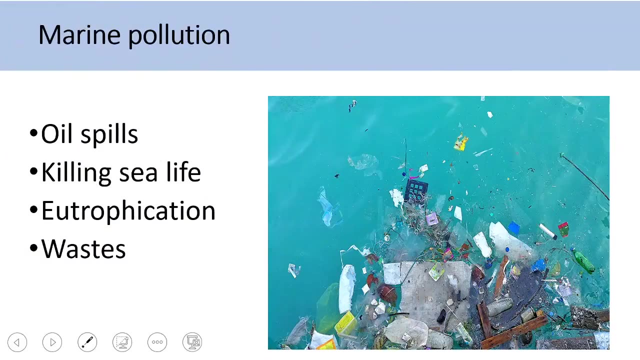 But in order to reach these minerals, you have to clear large areas of land on the surface of the earth, And clearing large surface area means clearing or destroying habitats in this area: Marine pollution, Oil spills from petroleum tankers, killing sea life. 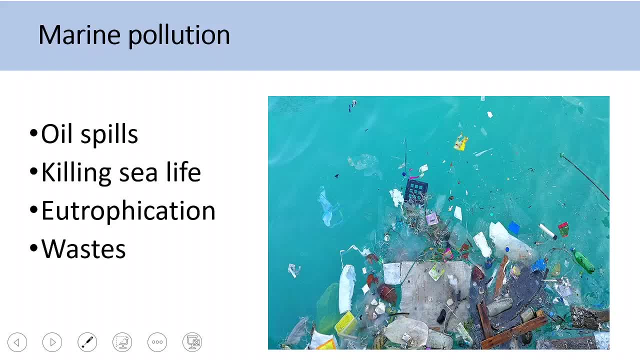 The fertilizers that leak from agriculture. using fertilizers end up with eutrophication. When these fertilizers leak to the water, allow algae to grow on the surface of water, preventing sunlight from reaching the plants in the seafloor. This means less oxygen in the water. 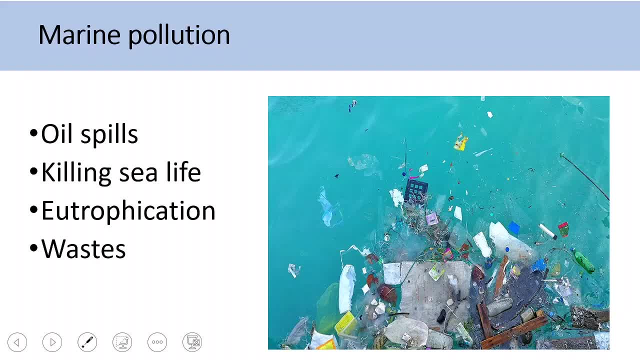 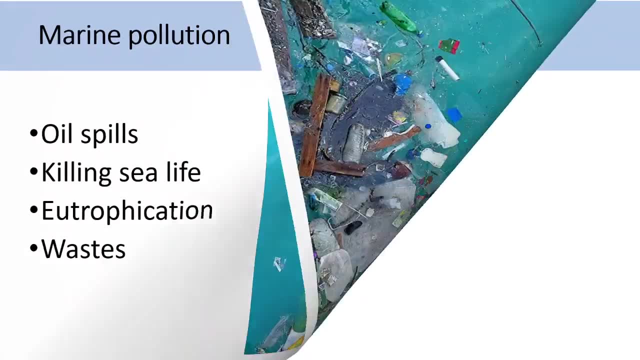 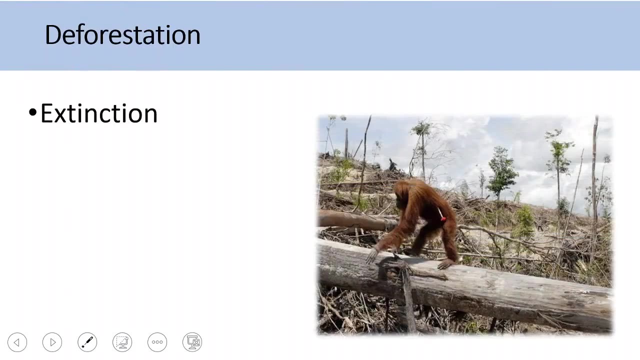 Marine animals will die. Also, throwing waste and garbage in the water destroy marine habitats. So let's talk now about deforestation, The huge negative impacts of deforestation, Deforestation on the environment, Extinction. So the first negative impact is extinction. 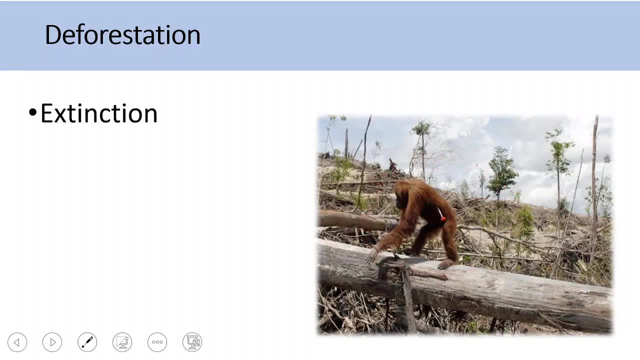 When you destroy the habitat for these animals. Now they don't have any other place to live, So they have two options: Either they die out or they migrate to a new place. If they cannot migrate and they cannot adapt, this means they will die out. 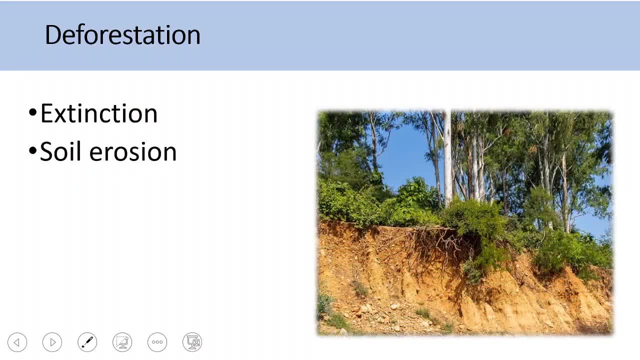 So this results in extinction. The second impact is soil erosion, The roots of the trees. The roots of the trees: They anchor the soil, And cutting the trees, this means nothing is holding the soil anymore And the soil can be easily eroded by wind or water. 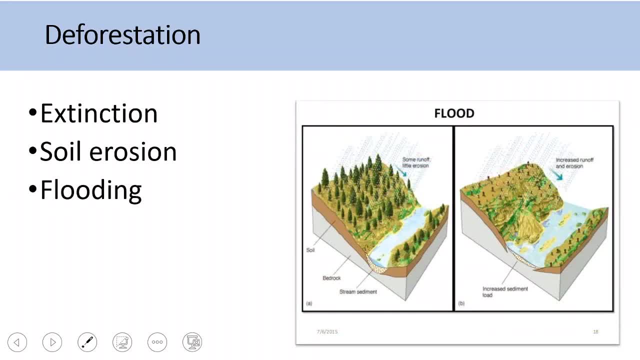 And cutting the trees. as we said before, the soil is not anchored by the roots of the trees. This means it will erode to the valleys. In addition, the soil now cannot retain water. It cannot absorb water properly, So the water will quickly run off into the valleys. 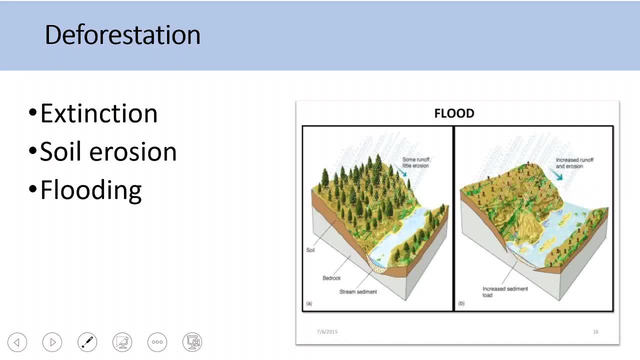 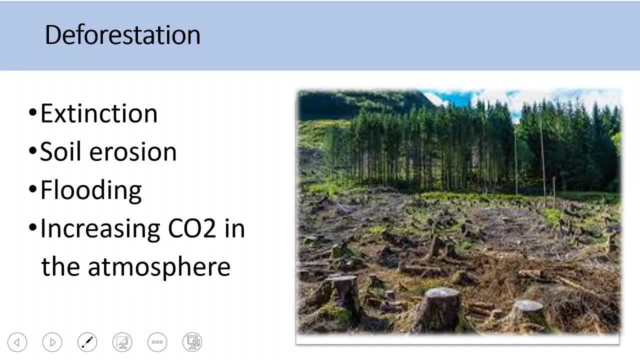 This will cause huge flooding to happen And- the last here- increasing carbon dioxide in the atmosphere. Trees absorb carbon dioxide from the atmosphere by the process of photosynthesis. This means that The only way, or the main way, for carbon to enter into living things and reduce from the atmosphere is by the process of photosynthesis. 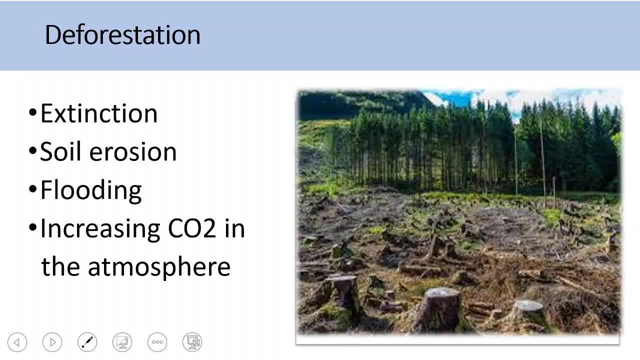 And cutting trees makes fewer trees or keeps only fewer trees that can absorb carbon dioxide, So now fewer trees are absorbing this carbon dioxide. We end up with more carbon dioxide in the atmosphere. It cannot be absorbed and this will lead somehow to global warming. That's all, Thank you.